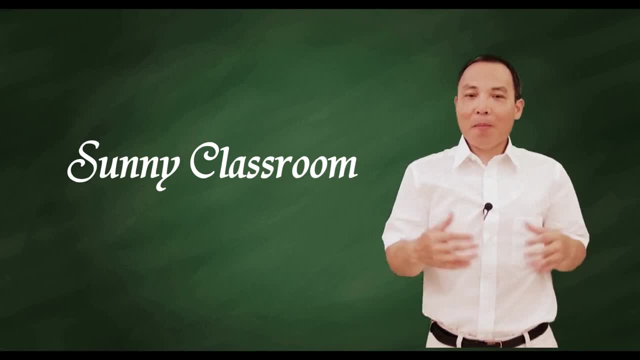 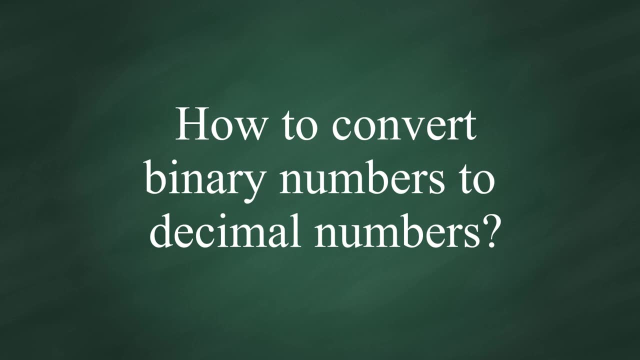 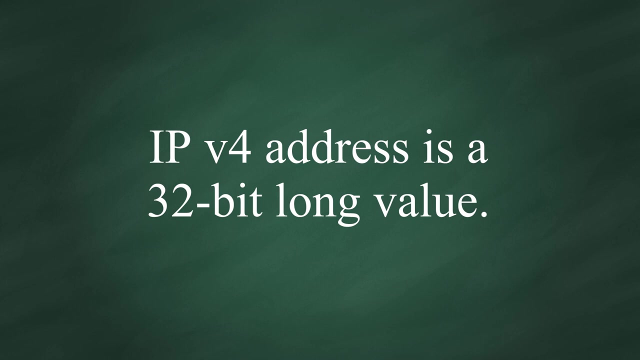 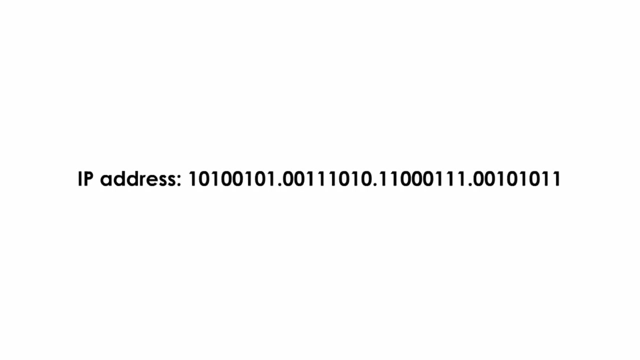 Hello, and this is Sunny. Welcome back Today. my topic is how to convert binary numbers to decimal numbers. in terms of IPv4 address, IP address is a 32-bit long value. Now let's look at this IP address in binary format. 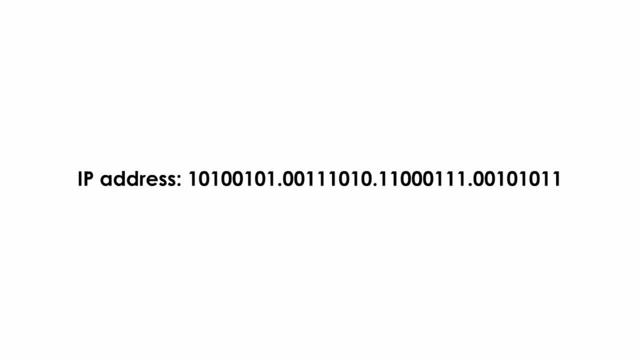 It is a 32-bit long string of zeros and ones. There's four sets or four groups of zeros and ones separated by dot. Each set is 8-bit long and that's why we call it an octet. Now let's convert this IP address. 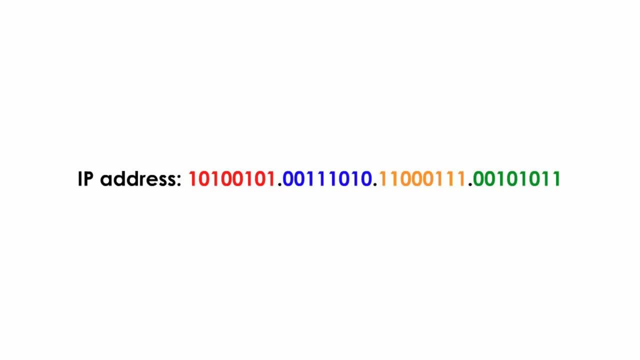 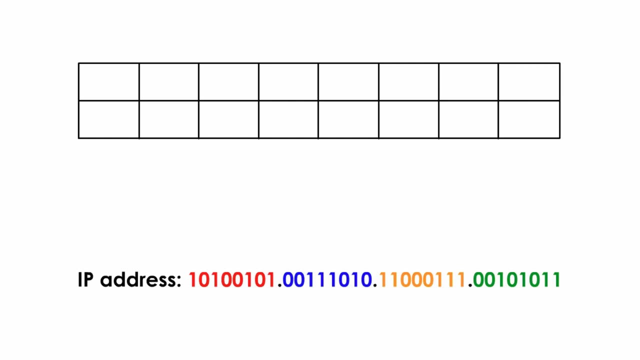 From binary numbers to decimal numbers. First, let's draw a two-row eight-column table, Starting from the right side, filling in the top row with eight numbers: 1,, 2,, 4,, 8,, 16,, 32,, 64,, 128.. 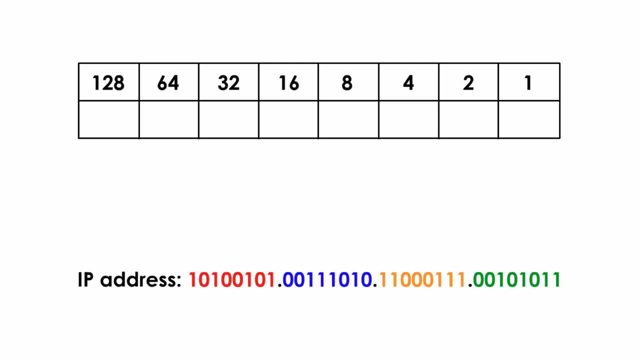 There's a pattern for this: eight numbers Starting with 1,. the next number is 2,, which is double 1.. 4 is double 2,, 8 is double 4, and 16 is double 8, and 32 is double 16, and 64 is double 32, and 128 is double 64. 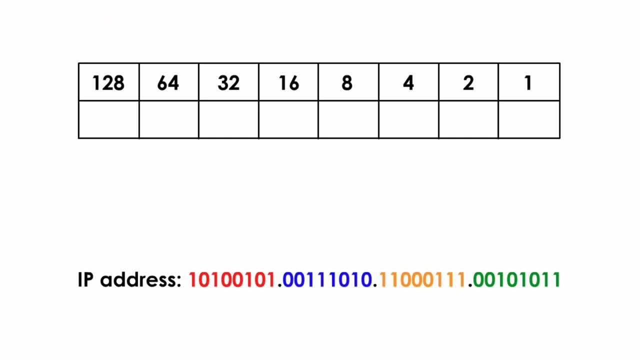 Let's call this table the binary table, because we will use this table in the following several videos. It's very useful. Let's convert these first 8-bit binary numbers, or the first octet. This is how it works. We put eight binary numbers to the binary table, from left to right, one by one. 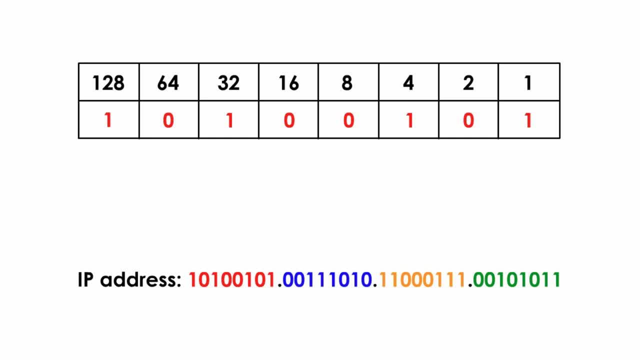 Making sure these eight binary numbers match their positions in the table. Now we look at ones only ignoring zeros. There's four ones in the second row. There's four ones. The next step is bring down the numbers above the one. They are 128,, 32,, 4, and 1.. 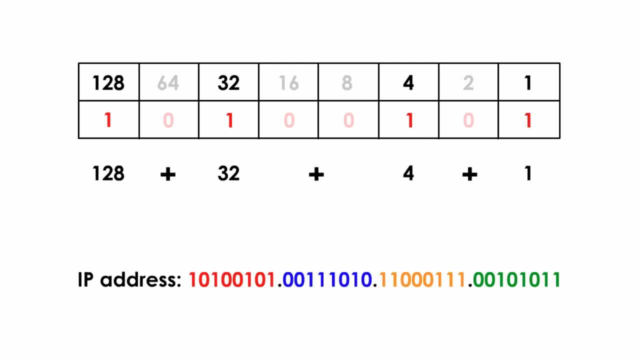 Then we add them up: 128,, 32,, 4, and 1.. And 28 plus 32 plus 4 plus 1, we got 165, that's it. The first octet is 165 in decimal value. 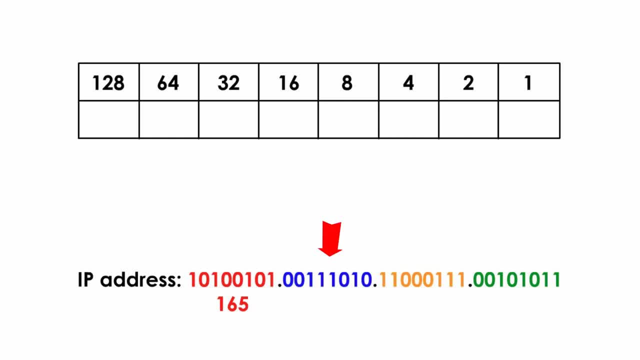 Let's convert the second octet, the second group. We put eight binary numbers to the binary table, One by one. We look at the ones, only ignoring zeros. We bring down the numbers above, the ones Which are 32,, 16,, 8, and 2.. 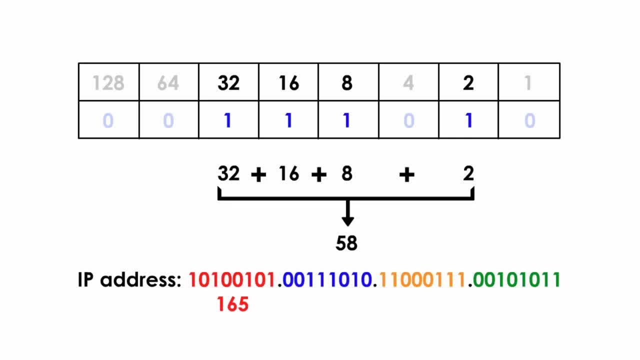 We add them up and we got 58. Thus the second octet is 58 in decimal value. Let's do the third octet. third octet: We repeat the same process by putting the eight binary numbers to the binary table one by one. We only look at the ones and bring down the numbers matching ones. 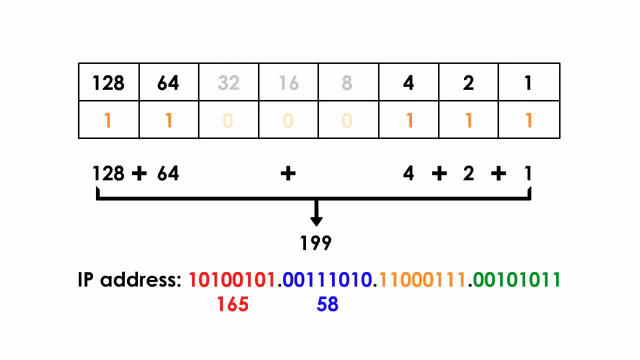 We add them up and we got 199.. That's the third octet in decimal value. Now let's finish the fourth octet. We repeat the same process. We only look at the ones, ignore all zeros and bring down the numbers above ones which are 32,, 8,, 2, and 1.. Adding them up, we got. 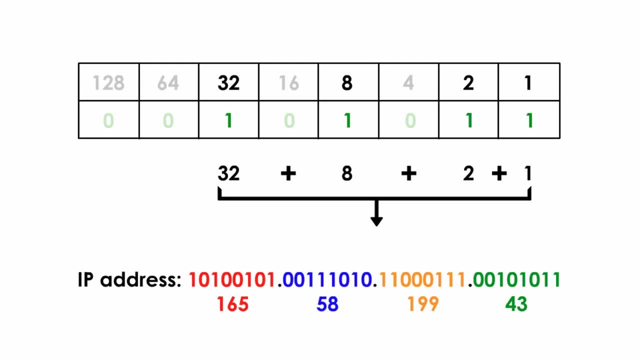 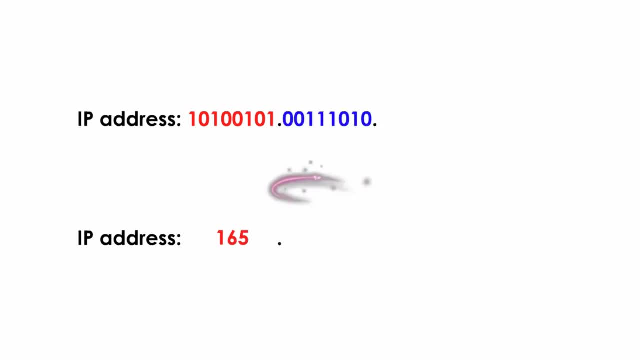 43.. Thus this IP address in ones and zeros is converted into IP address with more human-friendly data. We format decimal values, which is 165.58.199.43.. I hope this video is helpful and thank you very much and see you next time.